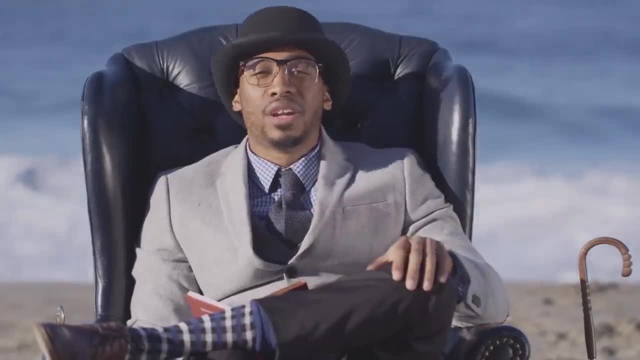 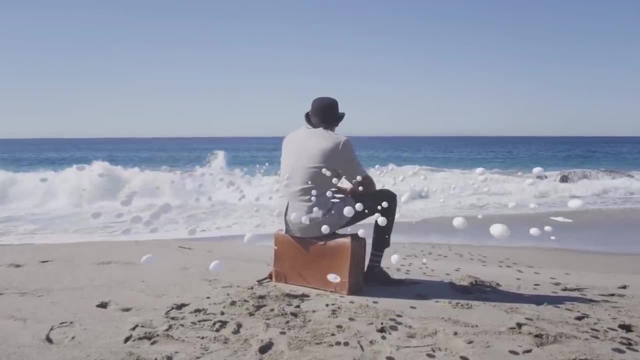 seconds, In an existence shorter than a vine video, we turn the circle of life Into our own personal conveyor belt. Somebody, anybody, help. We were given so much The only planet in this solar system with life. I mean, we are one in a million. No, actually, scientifically, 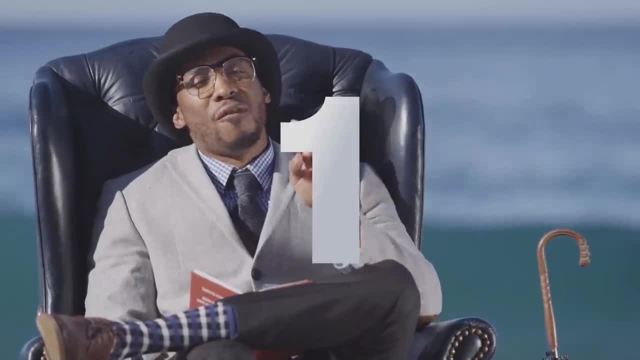 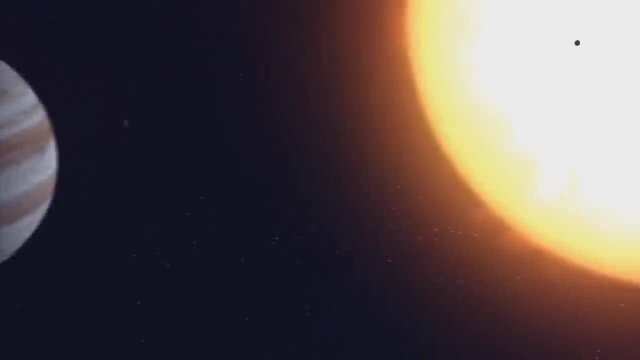 we are one in a billion, trillion. trillion, That's a one followed by 33 zeros, And I don't want to get too spiritual, But how? are we not a miracle? We are perfectly positioned to the sun so we don't burn, but not too distant So we don't turn to ice. Goldilocks said it best: We are just. 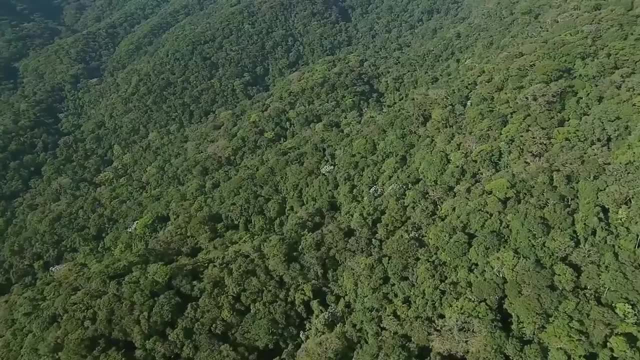 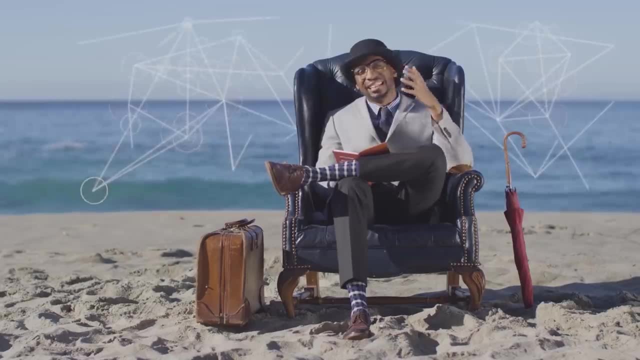 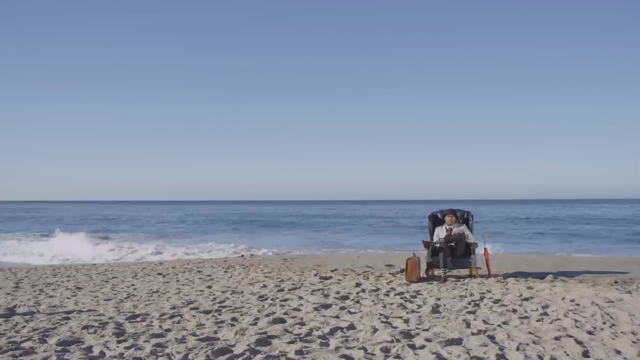 this paradise where we are given medicine from trees, not coincidentally but because, like the song says, we are family, Literally everything, every species is connected genetically, from the sunflower to the sunfish, And this is what we must recognize before it's too late, because the 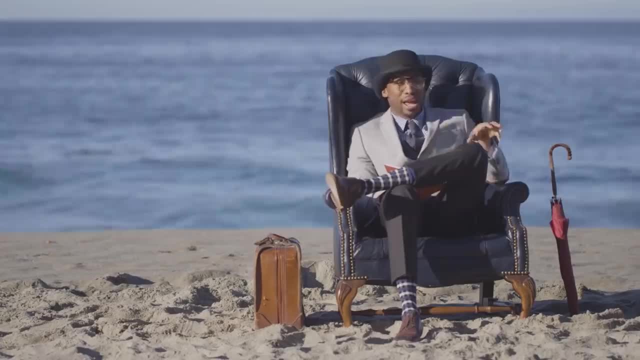 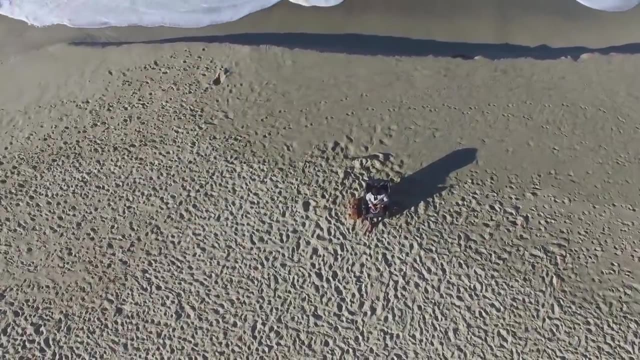 real crisis is not global warming, environmental destruction or animal agriculture. It is us. These problems are symptoms of us, byproducts of us. Our inner reflection, loss of connection, has created direction. We have forgotten that everything contributes to the perfection of Mother Nature. 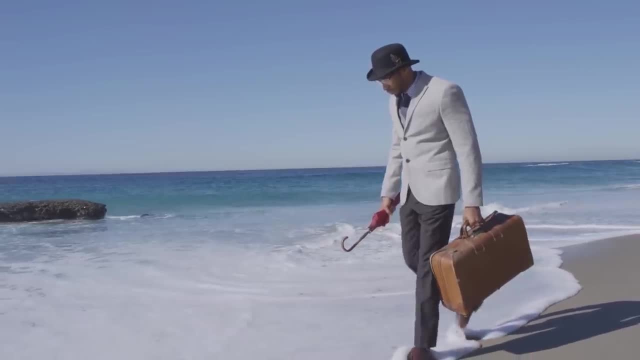 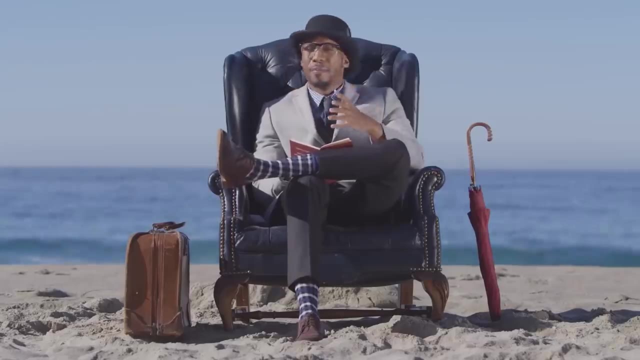 Corporations keep us unaware and disconnected, but they have underestimated our strength. Contrary to popular belief, millions are waking up out of their sleep, seeing our home being taken right up under our feet. We cannot allow our history to be written by the wicked, greedy and loony. It is our duty to. 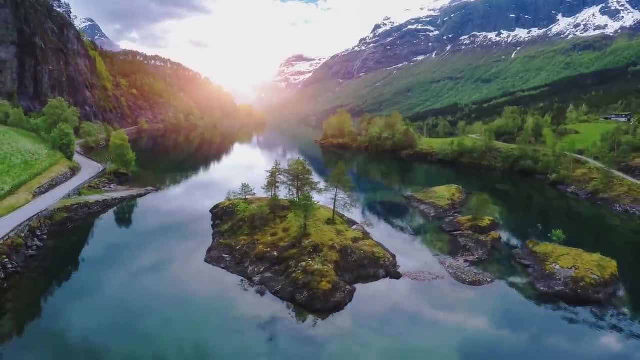 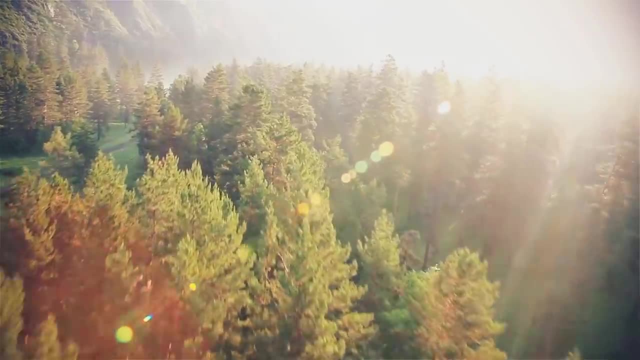 protect Mother Nature from those who refuse to see her beauty. Call me crazy, but I believe we should have the right to eat food that's safe, with ingredients we can pronounce. Water that is clean, Marvel at trees, Breathe air free of toxins- These are natural rights. 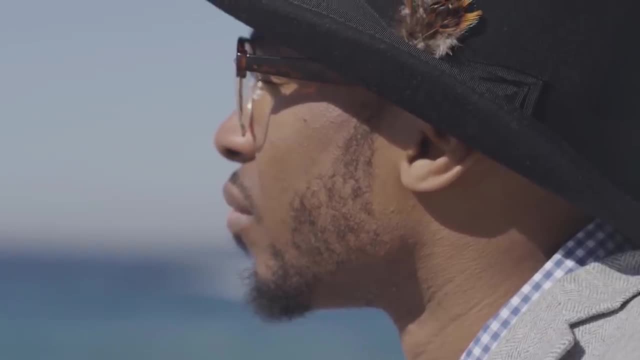 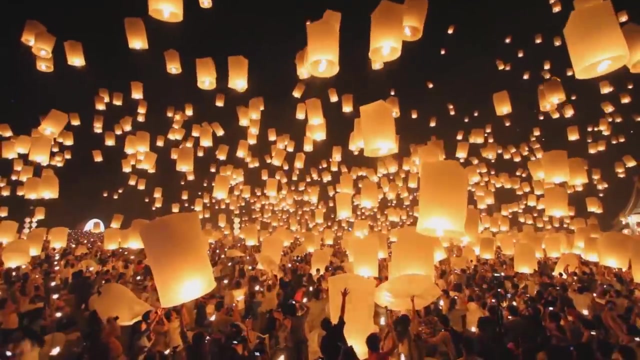 not things that can be bargained for in Congress. See, they want you to feel powerless, but it has been said that something as small as the flutter of a butterfly's wing can cause a typhoon halfway around the world. But when enough people come together, we too will make waves, and 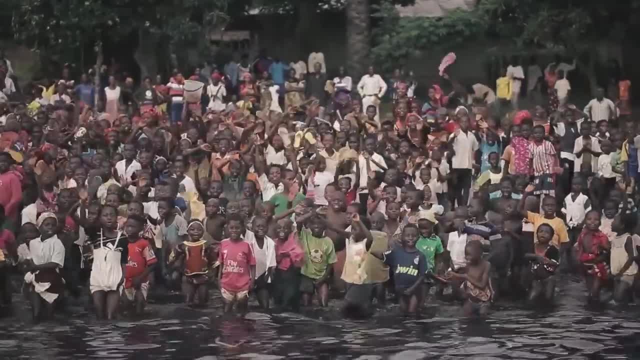 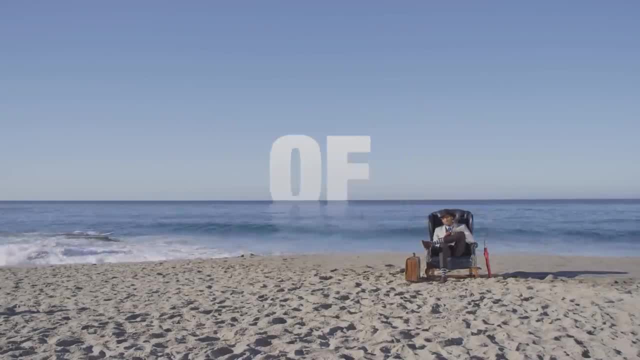 wash the world into a new era filled with love and connection, freedom for all, without oppression. But it is up to you- Yes, you watching this behind this screen- to make the effort, because time is of the essence and only together can we make it to the fourth second.